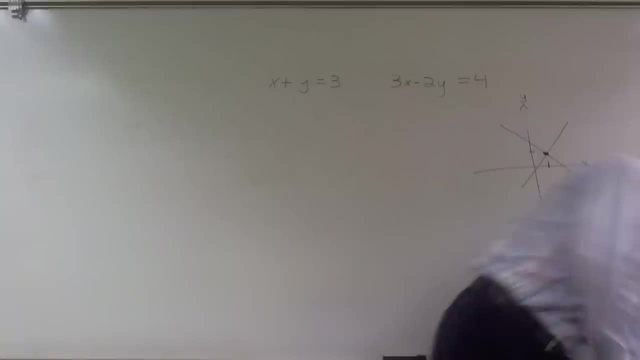 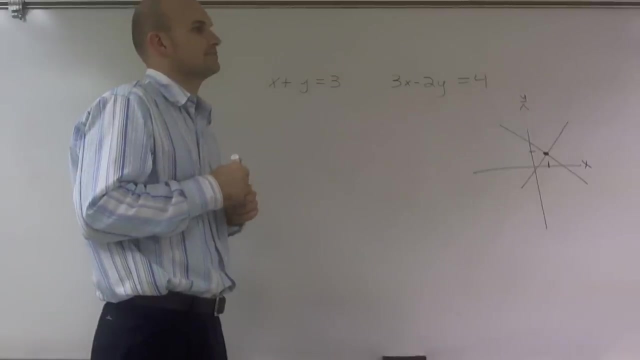 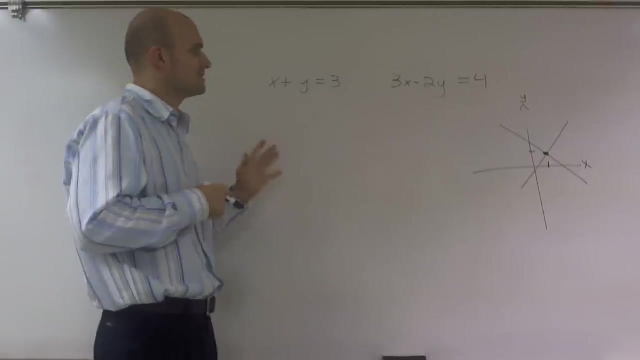 to the main office and not go to R9 for a question. Also, Officer Smith, would you please come to the conference room? Would you please come to the principal's conference room? Officer Smith, Okay, so then, to go ahead and figure this out, what we're going to have to do- 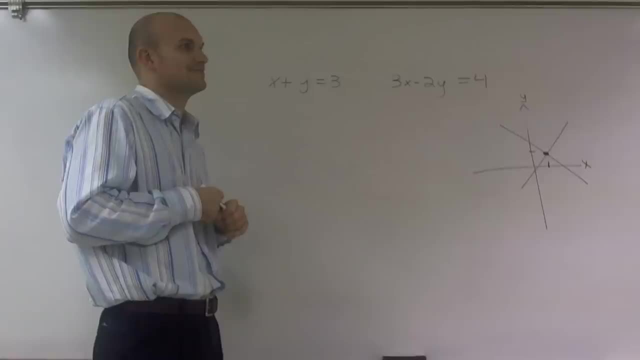 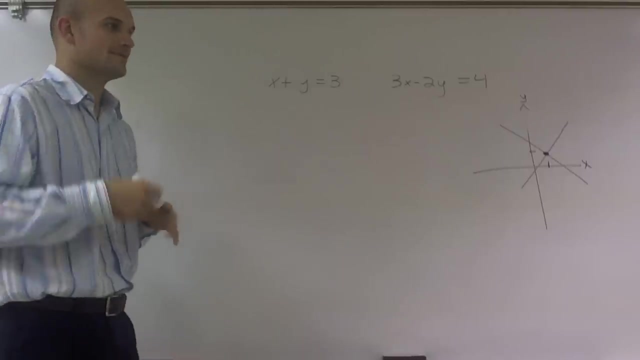 Video. Yeah, Just come by and say hi. I want to see what you're doing right now. Okay, We're doing intersections of two lines. Well, you can stay down. I'll be done with the video in two seconds, Thanks. 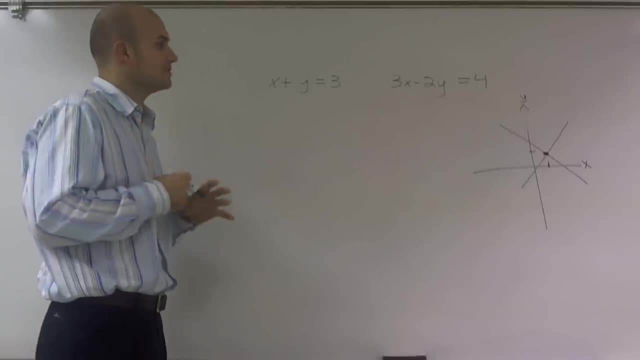 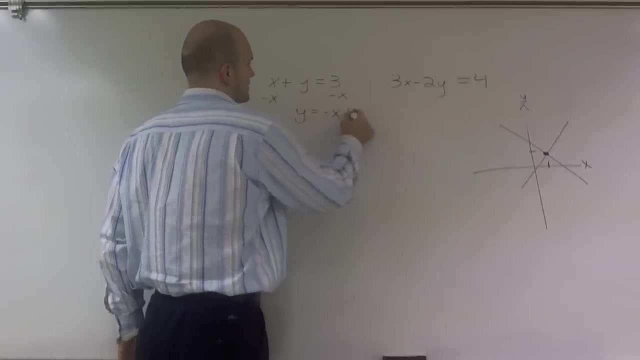 Thank you for showing me what you're doing. So then, what we're going to want to do is here: let's solve for y. So if I subtract the x on both sides, I get y equals a negative x plus three. Okay, So now, if I want to set these equal to each other, right, I want to. 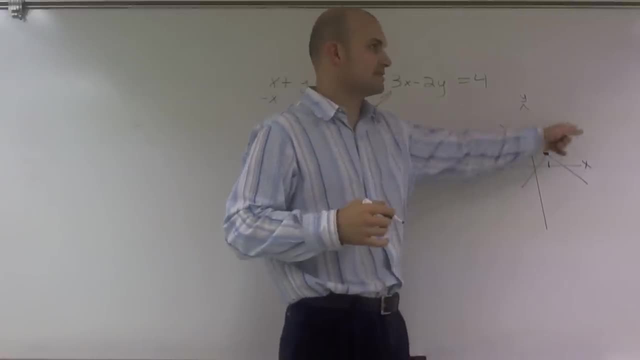 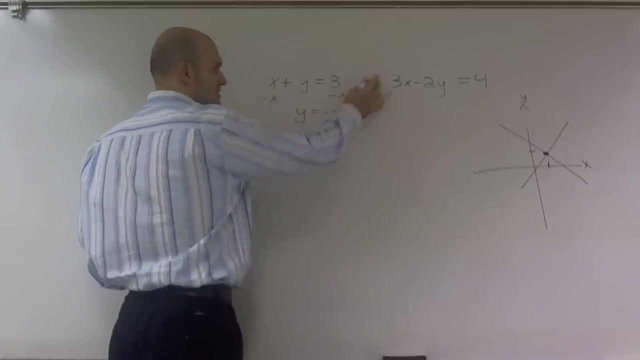 say: well, I know that my y values have to be the same for both of these equations. My two y values have to be exactly the same. So, therefore, what I'm going to do is I'm going to plug this equation into the other one, So I'll obtain three x. 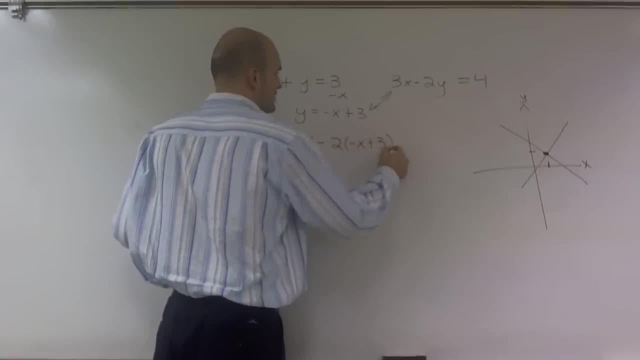 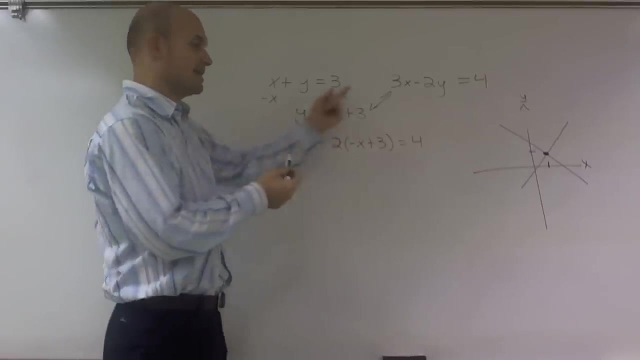 Minus two times negative. x plus three equals four. All right, Then, what I can do is, when the y values are the same, meaning I plug one y value into the other one I can find. when will the x values be the same? So I'll use distributive property to give me three. 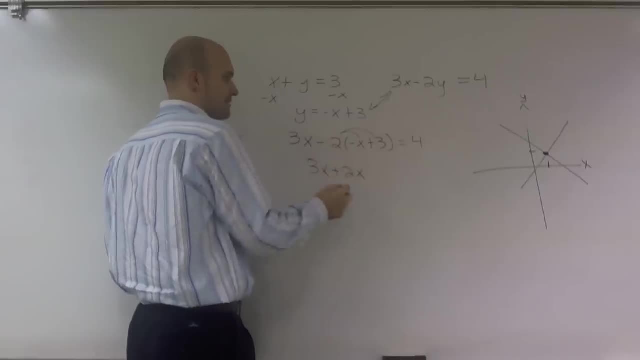 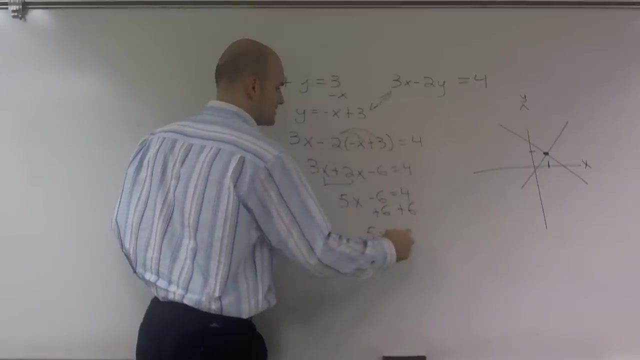 x plus a two x Negative. two times negative x gives you positive. two x Minus six equals four. Combine my like terms to give me five x minus six Negative. two times negative x equals four. Add six. Five x equals ten, Divide by five. 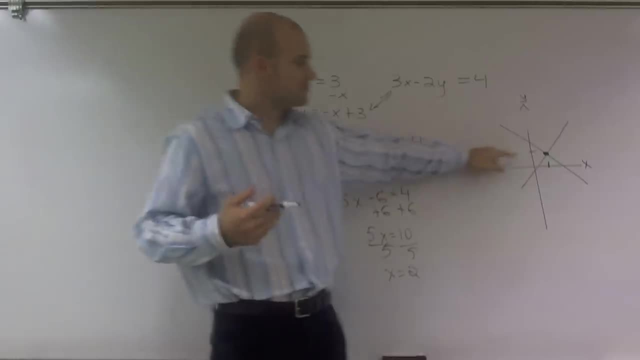 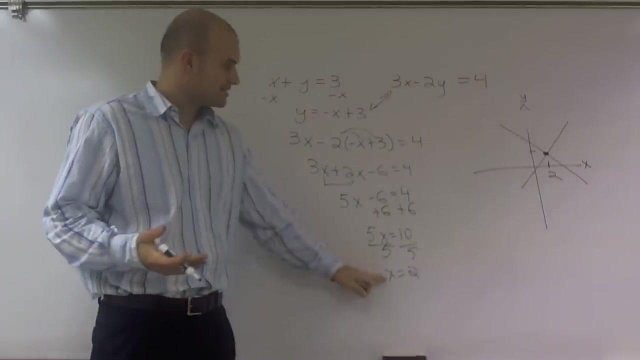 X equals two. So what that tells me is: when my y values are equal to each other, my x value is equal to two. So now the next thing I need to do is now: well, if x equals two, what is my y value for both those problems? So let's go ahead and take a look at that. 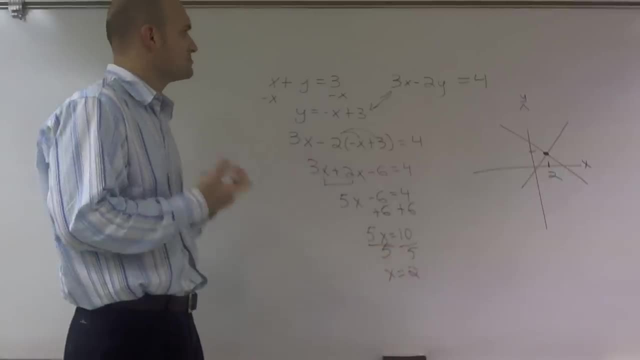 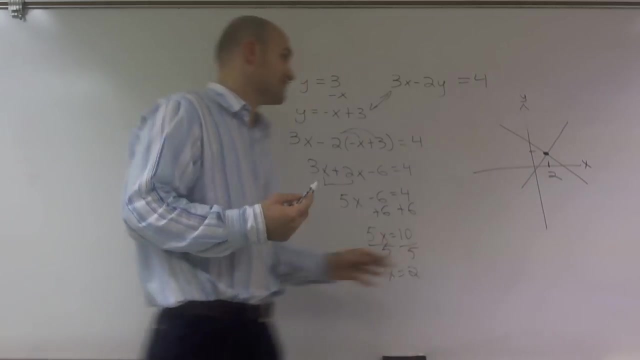 What I can do is I can plug two in for x and figure out what my y is going to be. So I'll plug it into both equations so you guys can see that when x equals two, my y values are going to be exactly the same, And then also we'll figure out what the y value is. So I